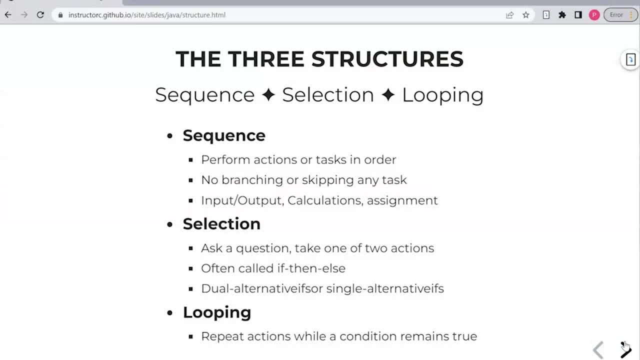 So there's three different structures: There's sequence, there's selection and there's looping. And so, with sequence, it's your input, your output. You may have a calculation statement, but it's essentially forming a task Selection. you come to a juncture in your program where you have to make a decision. 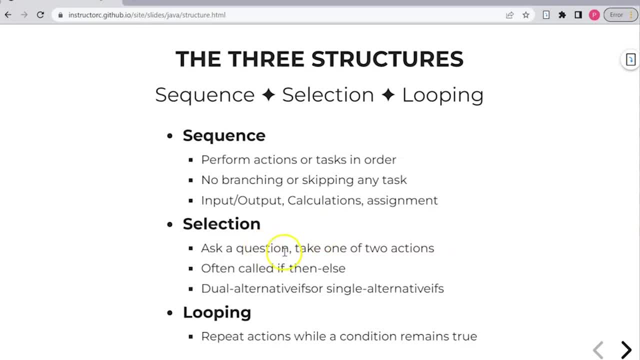 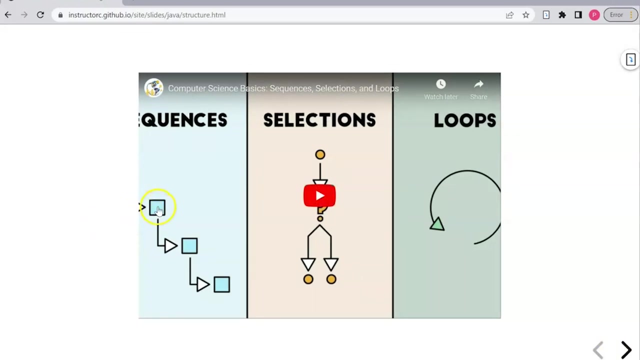 And so you will see structures such as if-else statements, if statements, Sometimes those are called single alternatives and dual alternatives, And then you have looping. You repeatedly do something until the condition Is met. Here's a video I would like you to take a look at that demonstrates each of the three different structures. 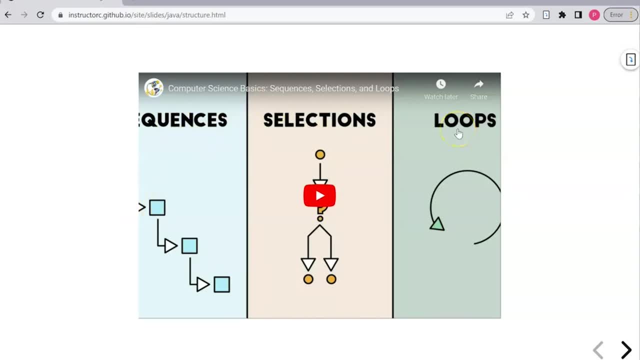 The sequence, selection and looping structures, And then we'll take a look at-give a visual and look at some code that would represent each of these three structures. All right, so hopefully that video gave you a little bit of context in terms of how those three structures can be used. 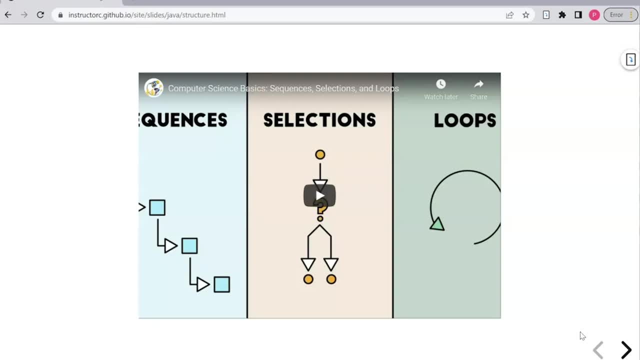 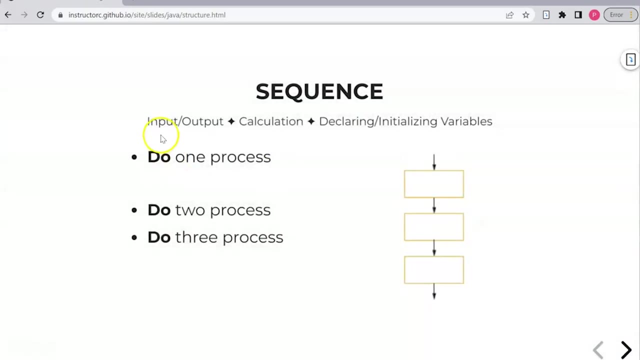 You can stack them, You can nest them And every application that you use, whether it's a website or a mobile app, a console application, you will find these three structures utilized multiple times within a program. So there's sequence Again: input, output, calculation. declaring variables would also be considered sequence, and initializing variables. 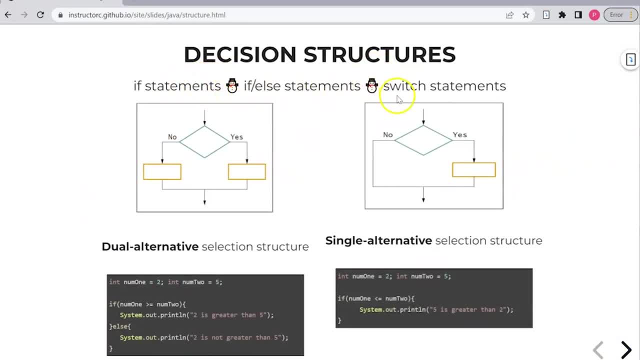 You have decision structures, if statements, if-else statements, And then these give you a visual of what that looks like, And so, especially if you're new to programming or new to learning how to code, working with a flow chart may be helpful to kind of see how the code functions and operates. 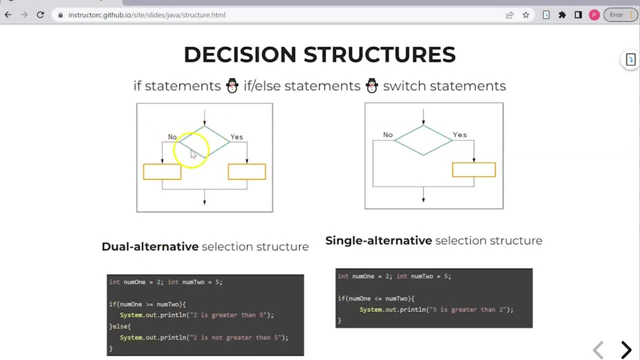 But then down here I also provide you with code and what that would look like. So this here is an if-else statement. So if this condition is true, yes, do this branch, Else, no, it's not true, Do this branch. 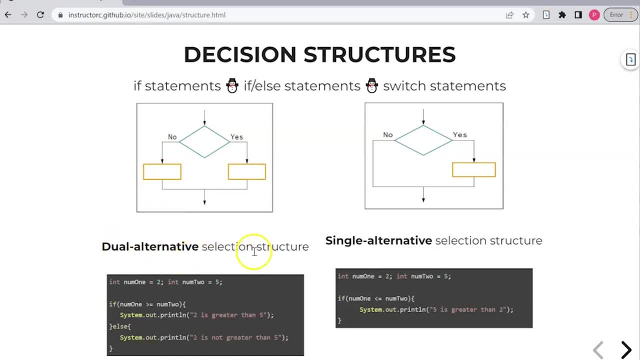 And sometimes we call it. it's what we call a dual alternative or a selection structure. The next structure is a single alternative. You have some condition. If this condition is met- yes, it's true, then do this branch, But there's no alternative. 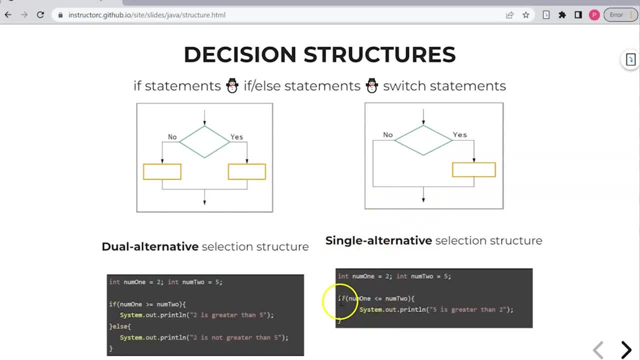 And so in this case it's a single alternative, And this is an example of the code. So if number one- num1, is less than or equal to num2, do this here, But there's no other alternative. Where versus the dual alternative, if this condition is true, num1 is greater than or equal to num2, say, 2 is greater than 5.. 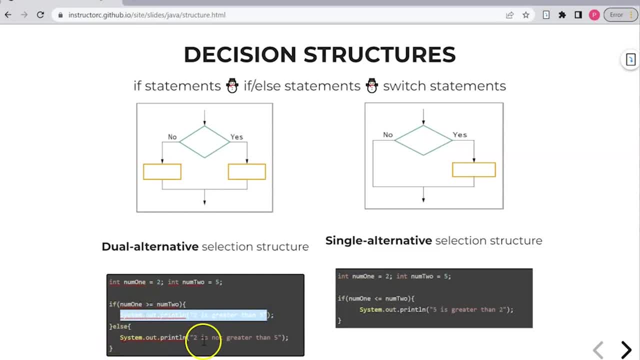 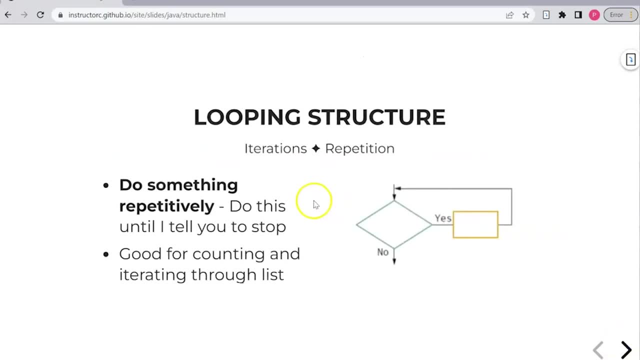 But if this condition is false, then it would output: 2 is not greater than 5.. Then you have the looping structure, where you want to do something competitively until the condition is met. And so here we ask the question: do this item in yellow until this condition is met? 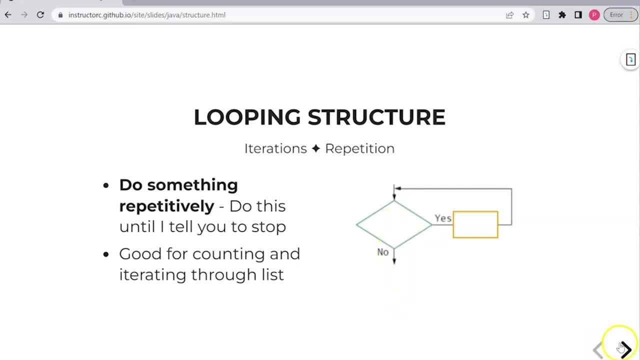 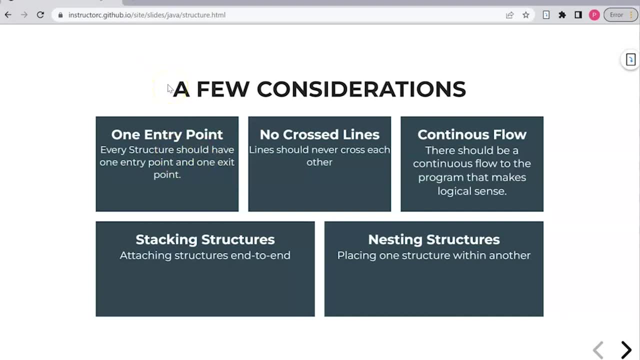 And then, once it's met, it continues on with the rest of the program. Here's a few considerations. One entry point, And this has to deal with making a well-structured program. One entry point: no cross lines, continuous flow, stacking structures, and you can also nest structures. 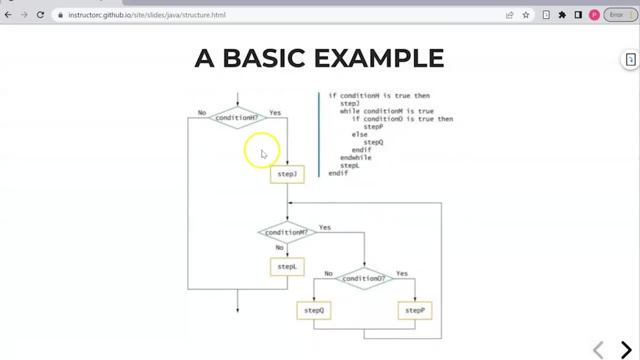 So here's an example of what that looks like. This is what we call a single alternative. So we'll have a condition, And this is also the pseudocode on the right here where my mouse is hovering. So if condition H is true, yes, 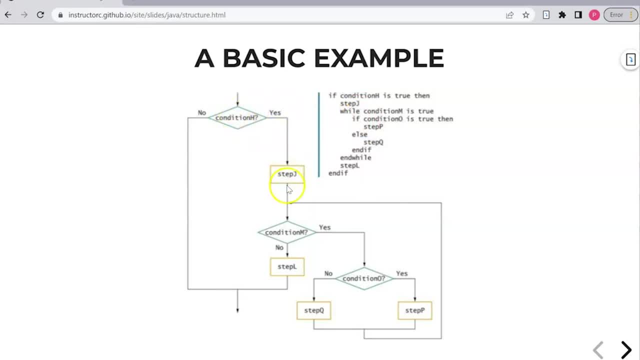 If you could say yes to that condition, do step J. So here we have single alternative, We have sequence, which is step J, And then here we have a looping structure. So if condition M is true, yes, We're going to go down and do a dual alternative selection structure. 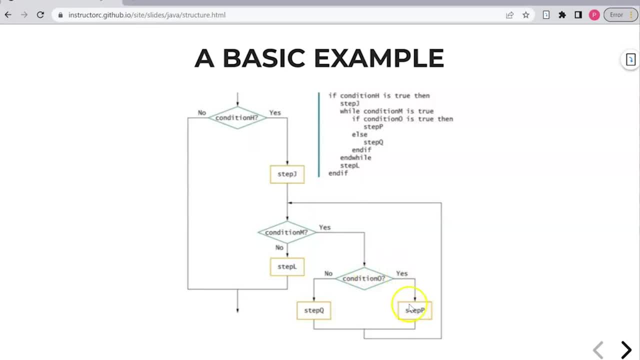 If condition O is true, yes, Do sequence step P. If condition true is not true, then we do the alternative, which is going to be step Q, which is a selection sequence structure, But then it continues to ask the question over and over until this condition M is met. 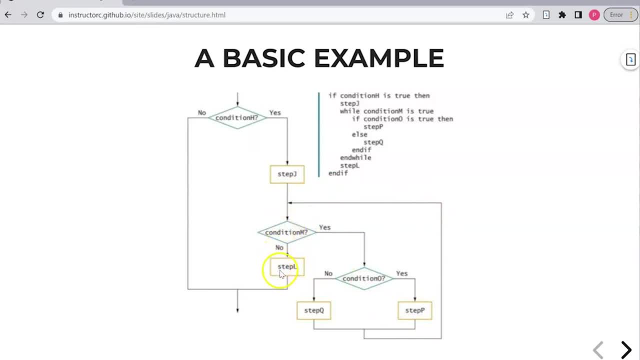 Once this condition is met, or once it's not met, then you go down to step L and then you go back to the overall structure and you exit. So you see all three structures at play here. You see the single alternative. You see the sequence with step J. 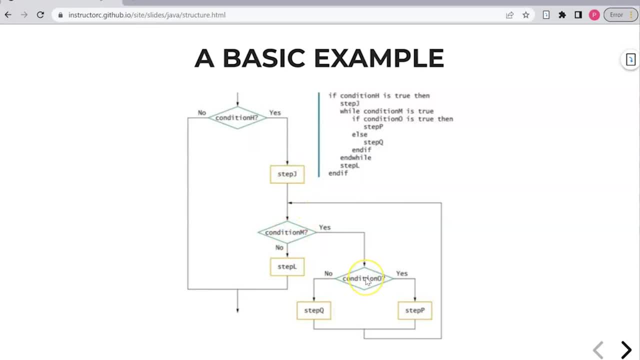 You see the looping structure, You see the dual alternative selection structure, But then also you'll see that these structures are nested within each other. So within the single alternative of condition H you have the condition M structure that's nested within this overall condition H structure or single alternative structure. 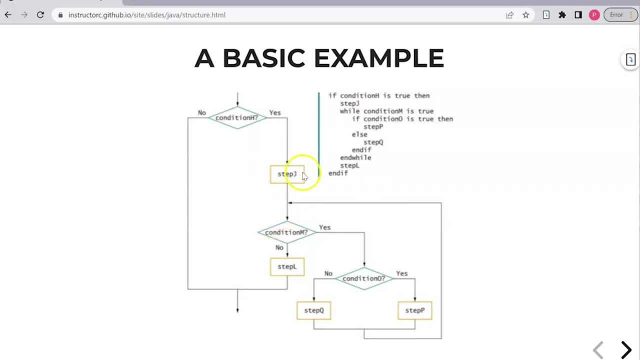 And this is the pseudocode that matches this code. here And again. this is helpful to think through and plan before you begin to write code. That way you know exactly how the program is going to function and operate before you begin to put the Java syntax in your source code. 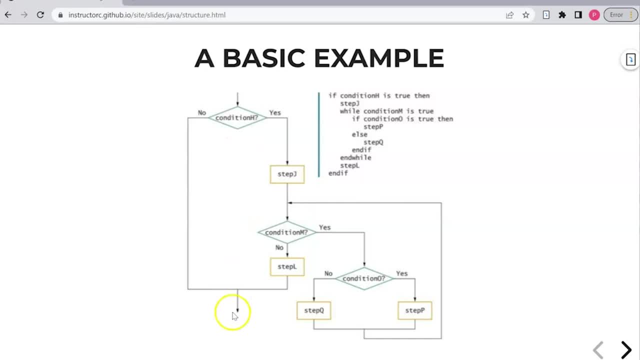 The other thing I want to mention here is that it's one entry and then one exit, And so we have one entry point here, where our mouse is hovering, and then one exit for this structure. Same here for our looping structure: One entry And then one exit. 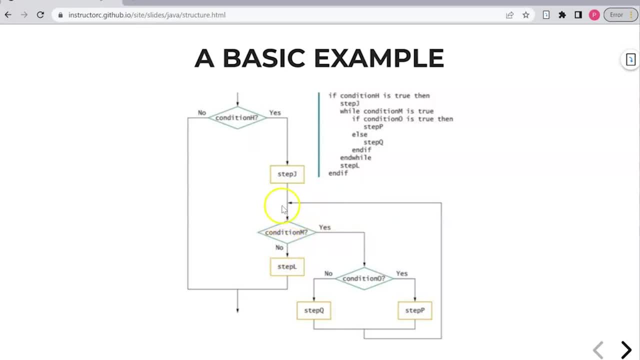 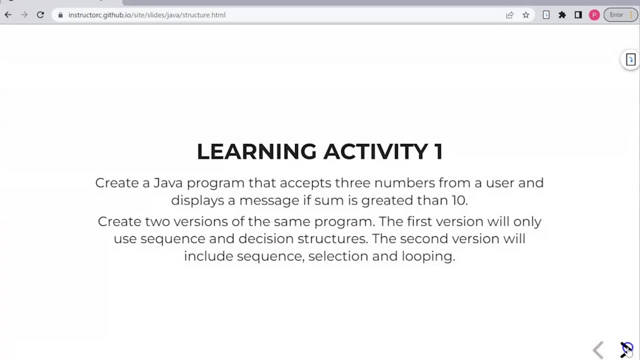 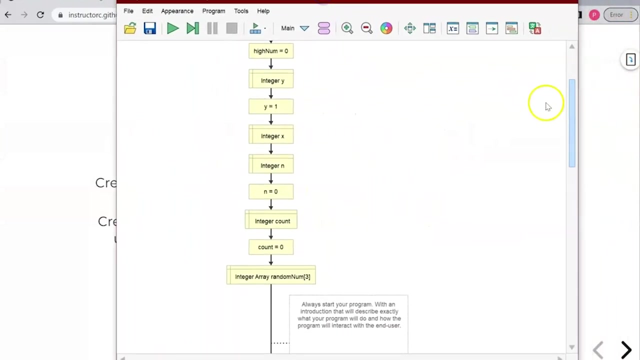 And then one exit, And so you don't have this line looking at the no branch right or crossing over to the no branch, And this will be considered a well-structured program. So here's a program that may be helpful. It's called Flogarhythm. 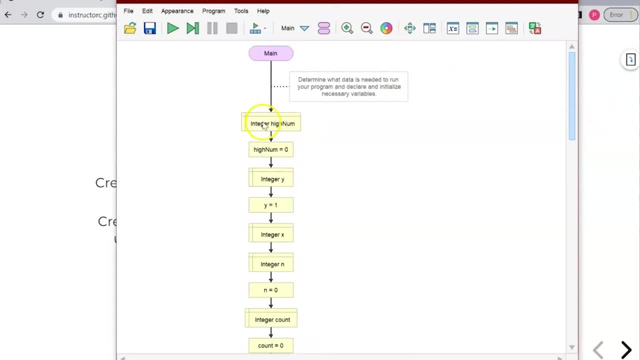 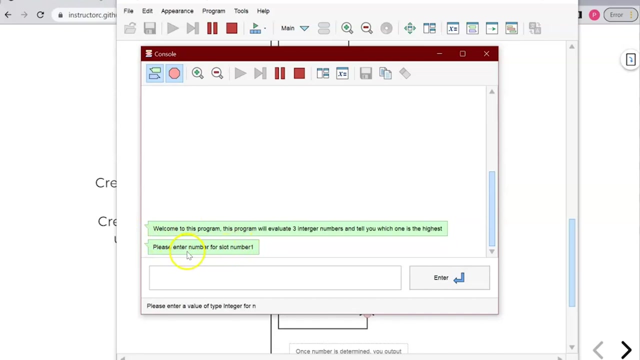 And it uses these shapes. So here's sequence. And what this program does is it allows the end user to input three numbers And it'll give the output the highest number of the three that you entered. So if you run this program, we have some sequence. that welcomes us to the program. 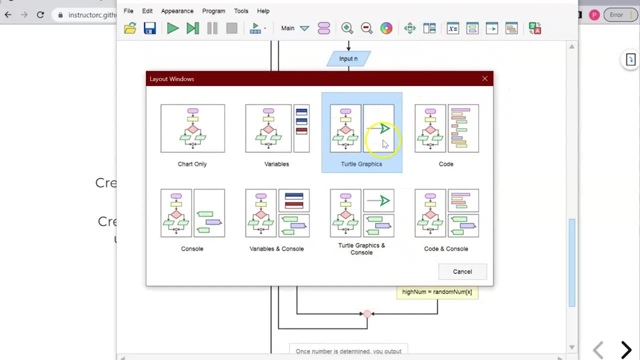 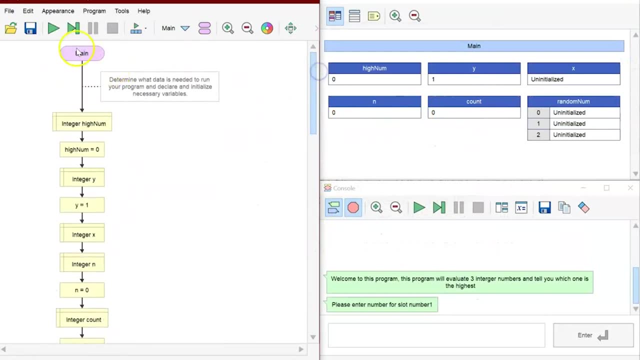 What I'm going to do is actually I'm going to do a different view here. Let's do the variable end console so we can kind of see what happens. We'll start at the top, We'll run the program. You'll see that it'll step through. 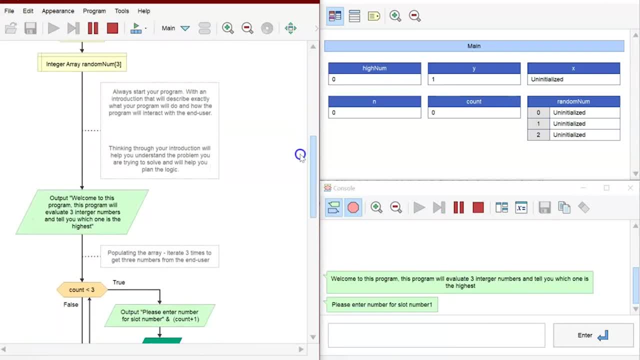 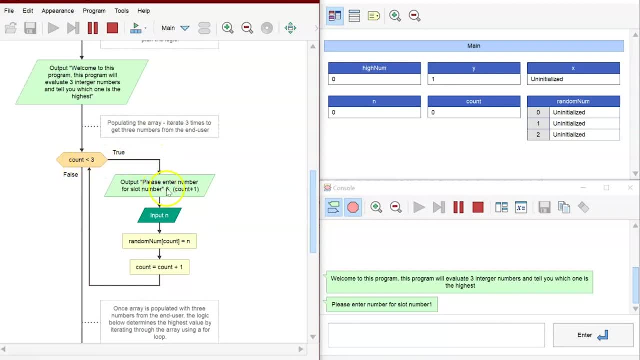 It basically declared our variables, initialized our variables, It did our output statement And then we go into our looping structure While count is less than three. here we have sequence, sequence, sequence, sequence. So you'll see that the variables are initialized. 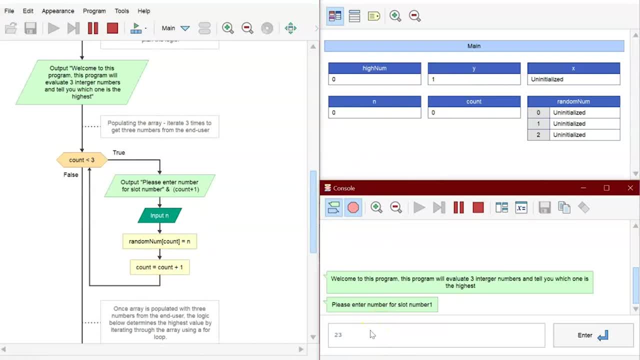 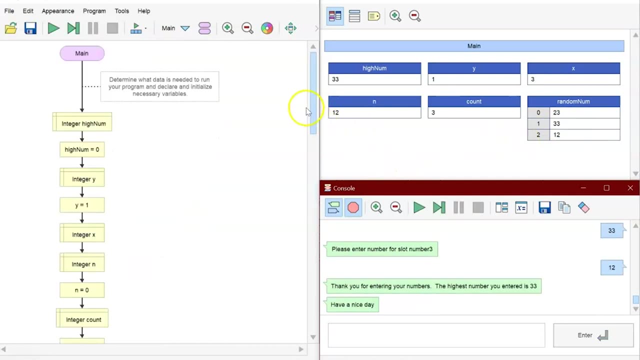 And we can go ahead and put a number for the, declare our first number in our random number array, We can do our second number And then we can do 12.. So this program executes and goes all the way through, all the way to the bottom here. 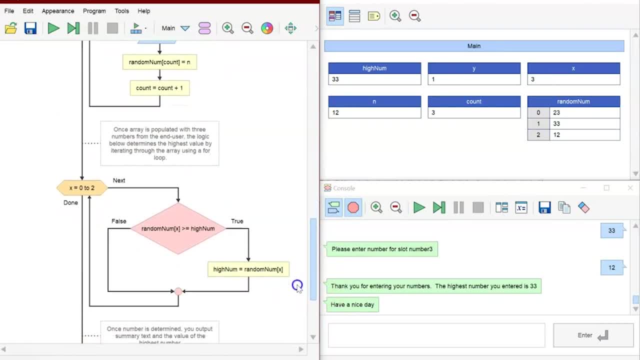 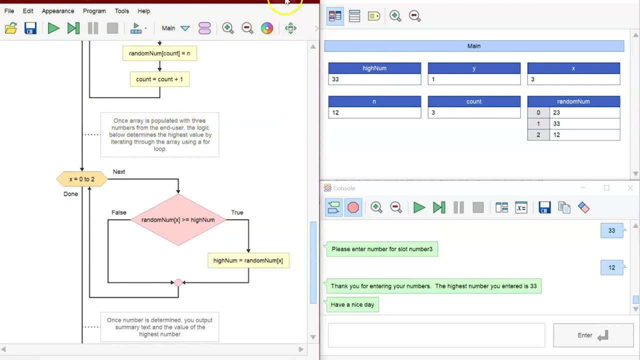 But you can see the various structures and how the program operates. There's a way that you can step through this slowly and see what happens. But nonetheless, this is Flogarhythm And it's a pretty cool program because it'll allow you to look at the pseudocode for this as well. 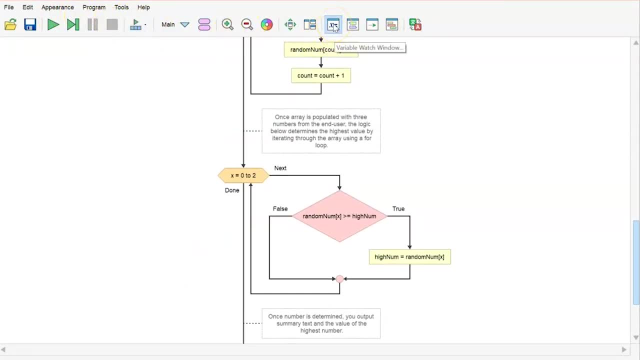 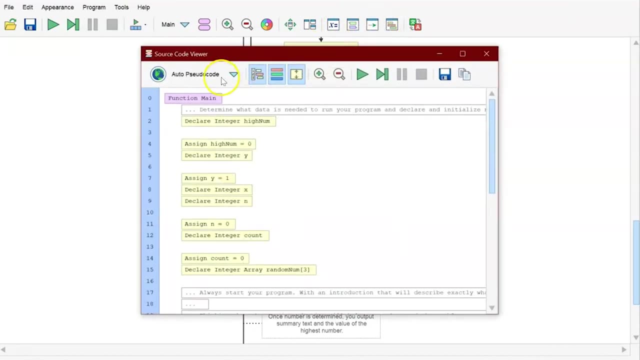 And I believe, if my research is correct, it'll show you the code for various languages. So this is a helpful tool. So, source code viewer, So it'll show you pseudocode And, if you want to look at it in Java. 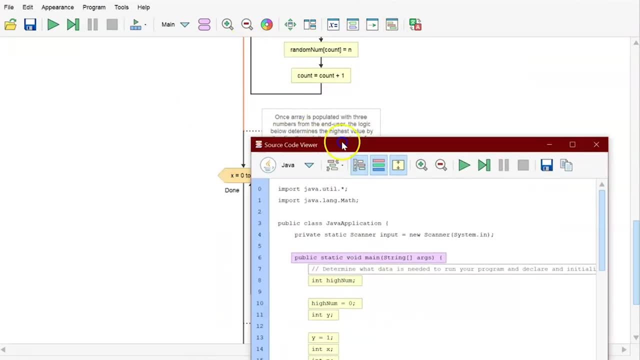 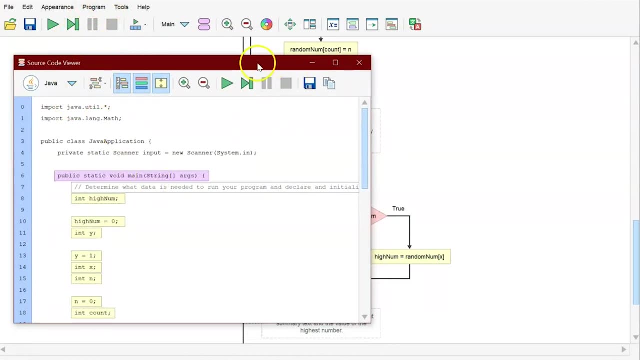 You can see what the code will look like in Java, based on how you place these structures And, actually, if this is a helpful tool, you may want to consider downloading it- It's flogarhythmorg- And begin to, I would say, run through the tutorial that is on the website in terms of how to use it. 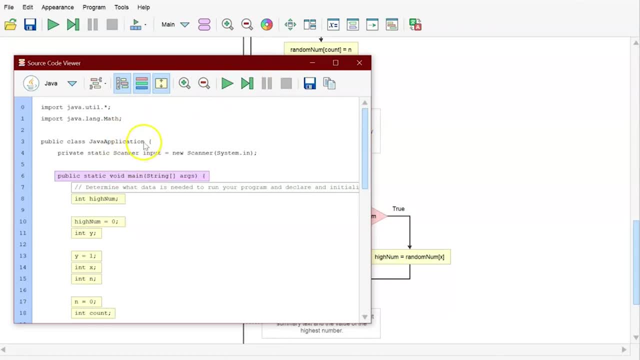 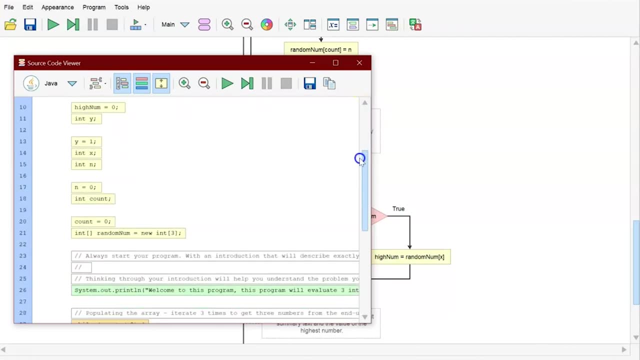 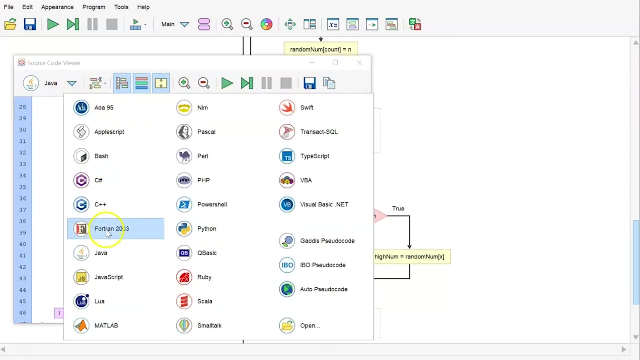 But it may be helpful in terms of planning out your programs and getting a visual of how the program functions before you actually write the code. So yeah, this gives you the code here in Java, But also it'll spew out the code in different languages. 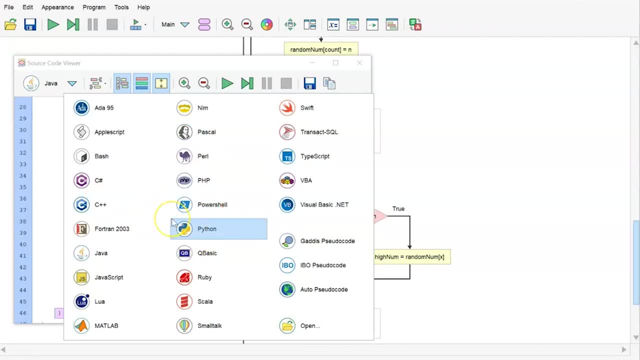 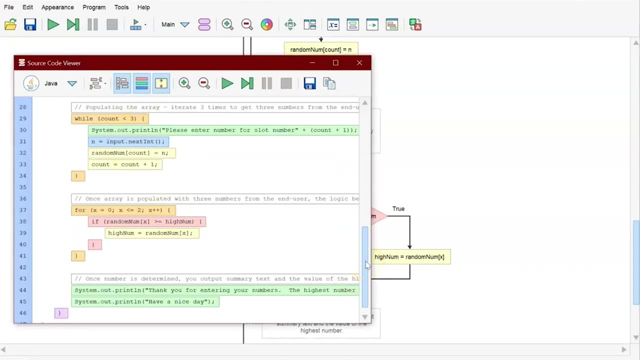 So if you're looking at Python or Java, it does some finagling of the code to get it to work, But for the most part you can get a good idea of the structures applied to different languages. So all right. So hopefully this video is helpful in terms of understanding how we can visualize our code and use the three different structures. 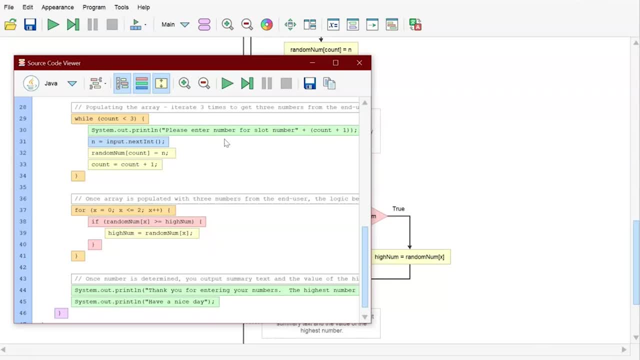 Sequence selection and looping To plan out our program and basically see how those particular structures are nested and stacked to create a full, exhaustive program. Stay tuned for the next video.